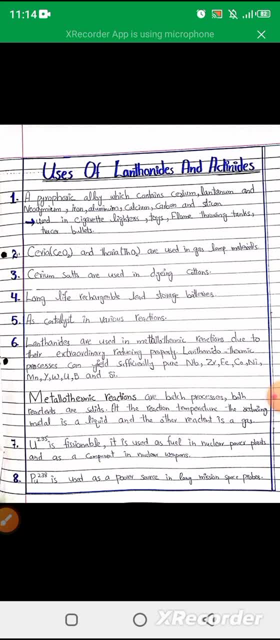 Number one: a periferic alloy which contains cerium, lanthanum, neodymium, iron, aluminium, calcium, carbon and silicon Periferic materials. when they come in contact with air, they catch fire within five minutes. Alloy means mixture of two or more than two metal species. Lanthanides and actinides are an integral part of periferic alloy. On the basis of this nature, periferic alloys are used in cigarettes, lighters, toys, flame throwing, etc. 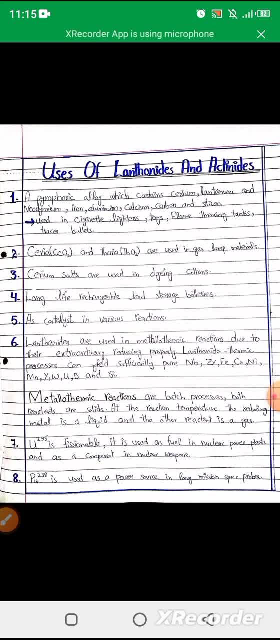 Number two, a periferic alloy which contains cerium, lanthanum, neodymium, iron, calcium, carbon and silicon. This is a fantastic use of lanthanides and actinides. For example, in nuclear reactions they are used as starting material for production of energy. Alloy means mixture of two or more than two metal species. Lanthanides and actinides are an integral part of periferic alloy. On the basis of this nature, periferic alloys are used in cigarettes, lighters, toys, flame throwing, etc. 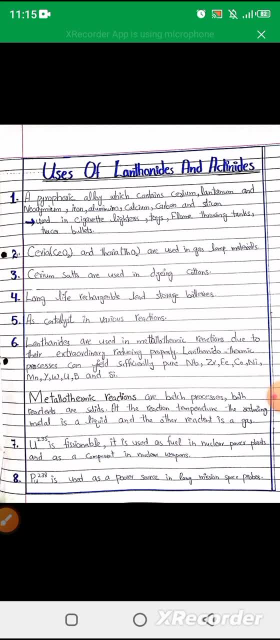 Number three: a periferic alloy which contains cerium, lanthanum, neodymium and silicon. Alloy means mixture of two or more than two metal species. Lanthanides and actinides are used in cigarettes, lighters, toys, flame throwing, etc. 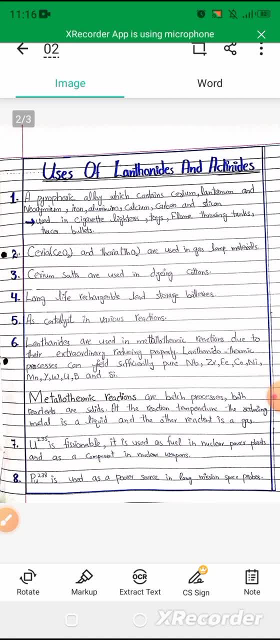 Due to their extraordinary reducing properties, lanthanides' thermic processes can yield sufficiently pure zirconium, iron, cobalt, nickel, manganese, uterine, tungsten, uranium, boron and silicon. Now we will discuss about metallothermic reactions. Metallothermic reactions are batch processes. Both reactants are solids at the reaction temperature. The reducing metal is a liquid and the other reactant is a gas. They are actually productive. 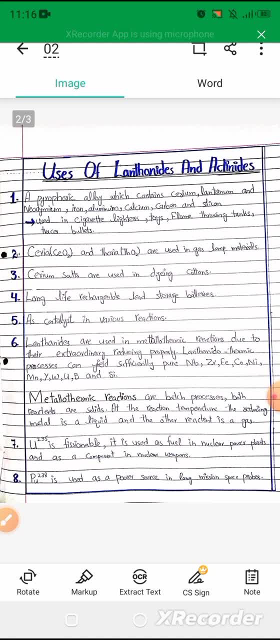 Number seven. uranium-235 is a fissionable. It is used as fuel in nuclear power plants and as a component in nuclear weapons. Uranium is a member of an actinide series and the atomic number is 92. It is the beginning of a series. Fissionable means natural disintegration Fuel in nuclear power plants. This can also be used for the production of thermal energy. 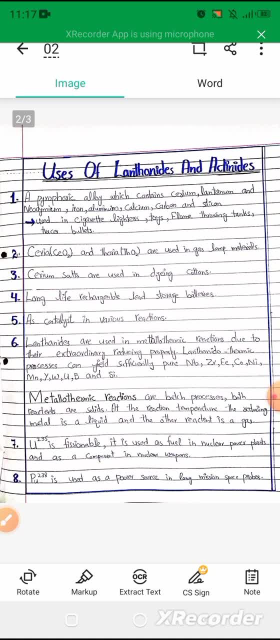 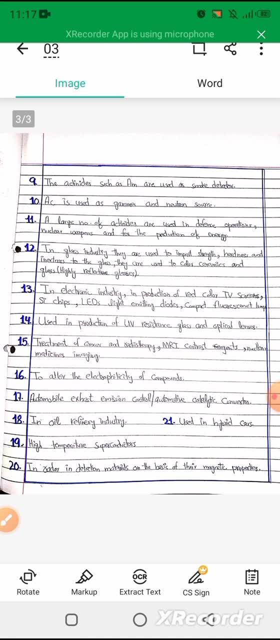 Number eight: plutonium-238 is used as a power source. Number nine: the actinides, such as americanium, are used as smoke detectors. Definitely, smoke detectors are instrumental in security. Number ten: actinides are used as a gamma and neutron source, So gamma rays and neutron rays are used for useful purposes. 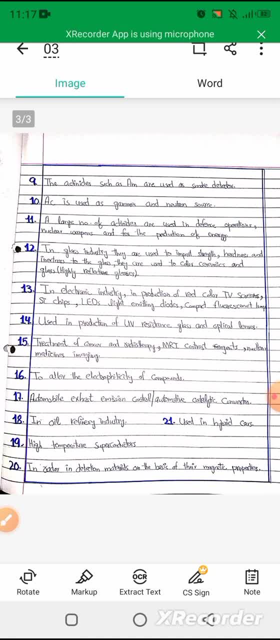 Number eleven: a large number of actinides are used in defense operations, Nuclear weapons and for the production of energy. Nuclear weapons can be used for destructive purposes. Production of energy can be used for constructive purposes. Number twelve: in glass industry, they are used to impart strength, hardness and inertness to the glass. They are used to color ceramics and glass. 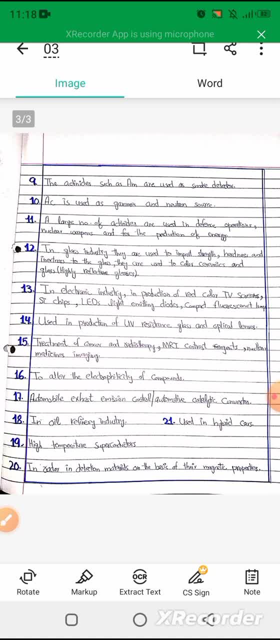 Hydrogen reflective glasses. Inertness and hardness can be achieved by actinides and lanthanides. Number thirteen in electronic industry industry in production of red colors, tv screens, silicon chips, leds, light emitting diodes, compact fluorescent lamp. in electronic industry. it also has certain applications that also is possible. 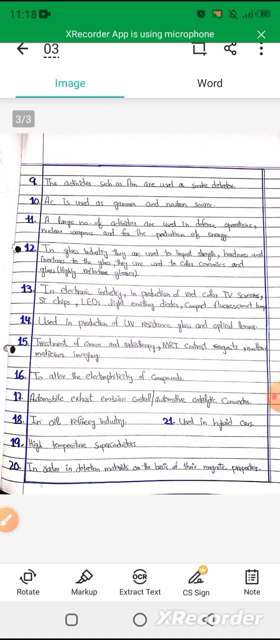 by actinides and lengthenides. number 14: use in production of uv resistance glass and optical lenses. so this is again useful use of actinides and lengthenides. number 15: treatment of cancer and radiotherapy, mrt contrast reagents, nuclear machine imaging. the most useful use of lengthenides. 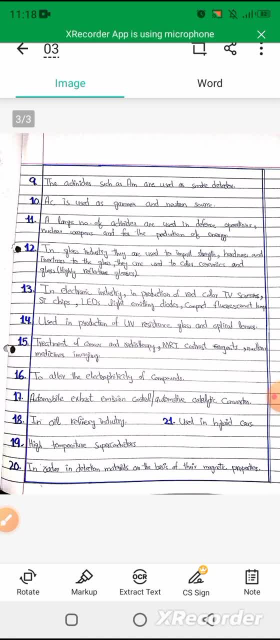 and actinides in the field of medicine is in use is in radiotherapy, number 16, the to alter the electrophilicity of compounds. they also use to alter the electronic properties. if you want to change electrophilicity of a compound in desired manner, then use actinides and lengthenides. 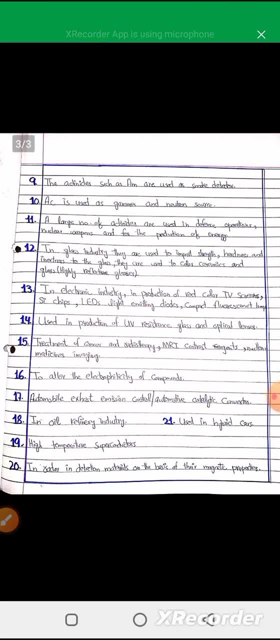 they also use to alter the electronic properties. if you want to change electrophilicity of a compound in desired manner, then use actinides and lengthenides. number 17: automobile exhaust emission control. this is used for the purpose of catalytic converter control. emission of.